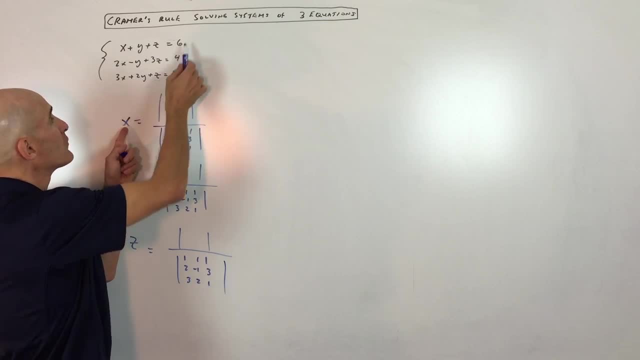 we're solving for x. we're going to replace the x coefficients with the solutions. so I'm going to put 6, 4 and 13, but then I'm going to put the remaining numbers here in the second and third column. okay, so you're with me so far. so all I did is I replaced the x coefficients with the solutions. 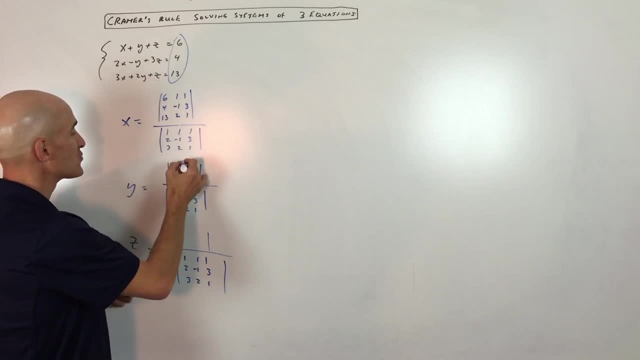 with y I'm going to replace the y coefficients with the solutions. so 6, 4 and 13. and with z I'm going to replace the z coefficients with the solutions. and then I'm just going to go back and you can see I'm putting the coefficients back in here: 1, 3 and 1. 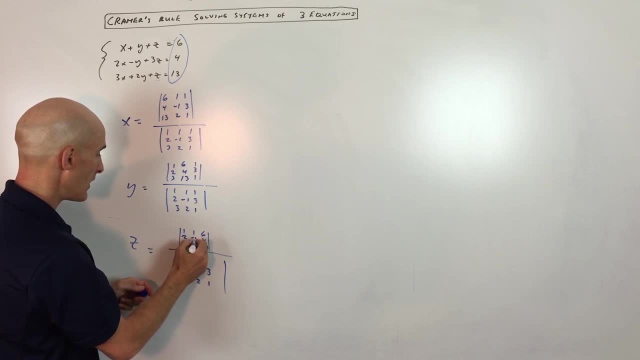 let's see here: this is going to be 1, 2, 3 and 1 negative, 1, 2. all right, so we've got it all set up. now, at this point, when you see these, you know bars like that. that means take the determinant. 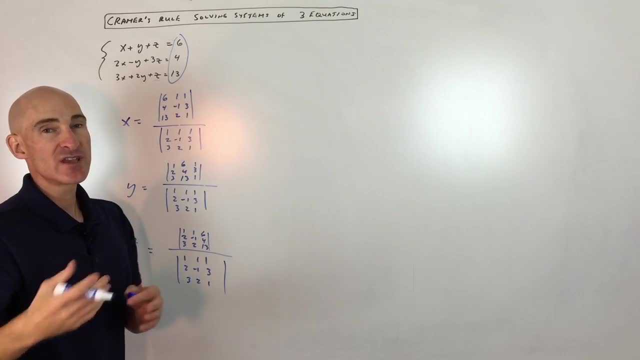 usually when you have a matrix, you'll have like a little bracket, okay. but when you take the determinant of a 3 by 3 matrix, there's a couple different ways to do it. I'm going to show you an easy way to do it, an easy way to remember it, and what you do is you just take the matrix and you. 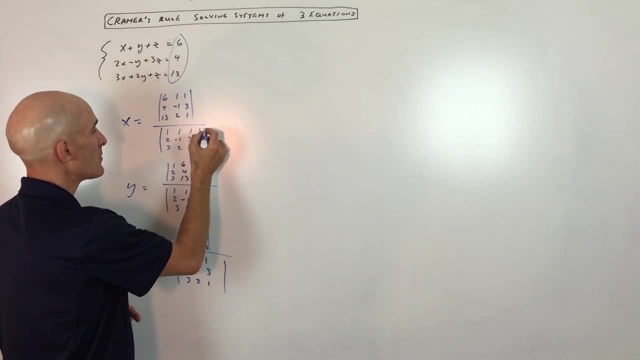 write it right next to the original matrix, so I'm just going to copy this down: 1 1, 1, 2. negative 1 3, 3, 2, 1. now what we're going to do is we're going to multiply in the diagonal like: 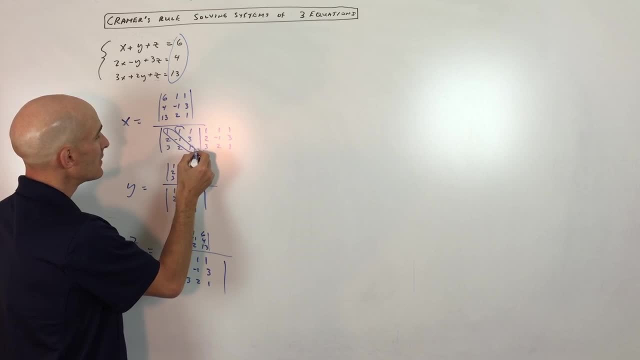 so so these guys multiply together, plus these guys multiply together, okay, plus these guys multiply together, so the ones going on the diagonal from this corner down to the right. so let's do that, so that's going to be negative. 1 plus 9 plus 4, okay, minus. 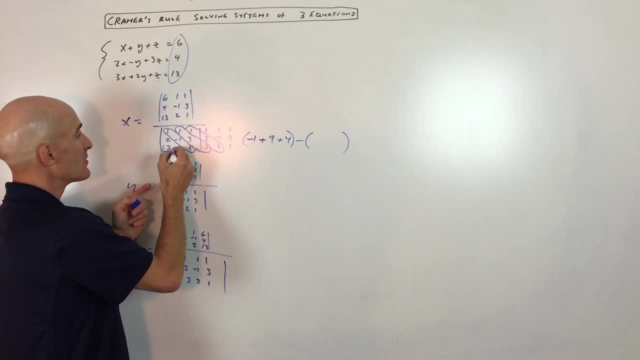 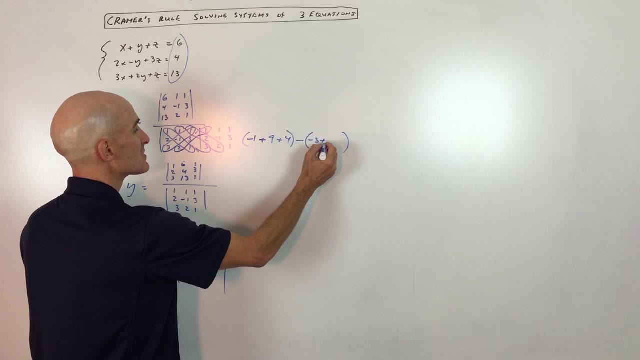 we're going to multiply the diagonals going up to the right, so this is going to be 3 times negative, 1 times 1, which is negative, 3, 2 times 3 times 1, which is 6, and 1 times 2 times 1, which is 2. so if 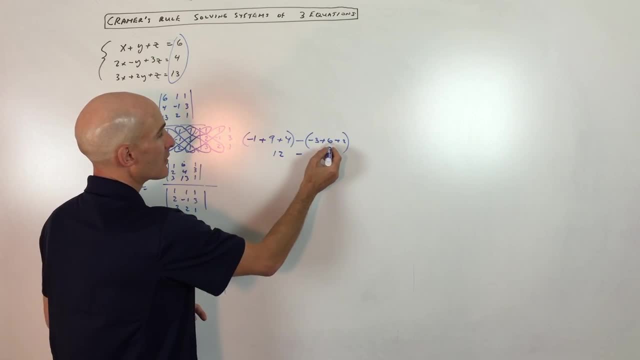 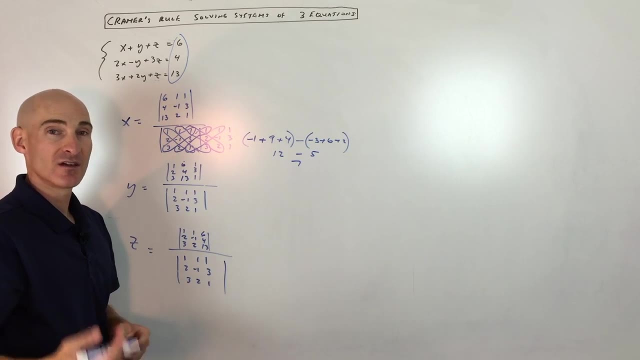 we simplify that down, we get: 13 minus 1 is 12. okay, this is 8 minus 3, which is 5, and 12 minus 5 is 7. so because the denominators for all three of these- x, y and z, these determinants, are exactly the same, 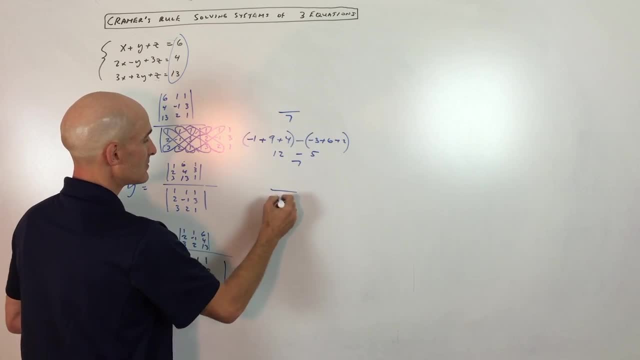 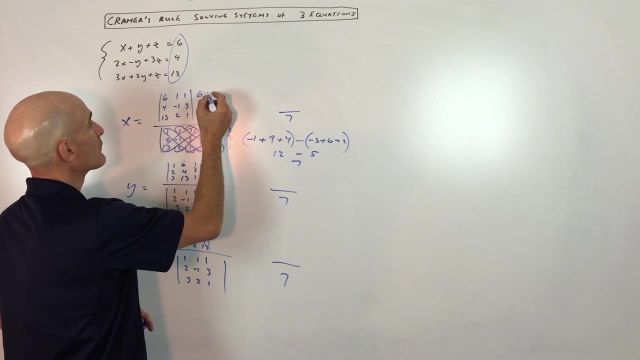 we know that the denominator is going to be 7, 7 and 7. are you with me so far? we're going to do the same thing with the determinant here. we're going to copy the first. you're going to copy the matrix right next to the original matrix. okay, so that's what I'm doing here. I'm just copying the matrix. 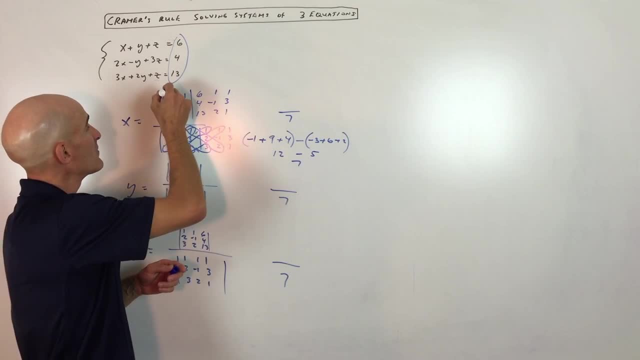 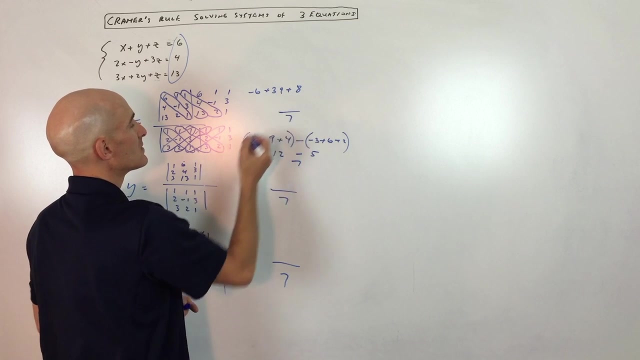 side by side, and I'm going to do the same process. I'm going to be multiplying on the diagonal, so that gives us negative 6 plus 1 times 3 times 13, which is 39. and then I'm going to do the same, plus 1 times 4 times 2, which is 8. okay, so that comes out to what here? let's see if we can. we'll. 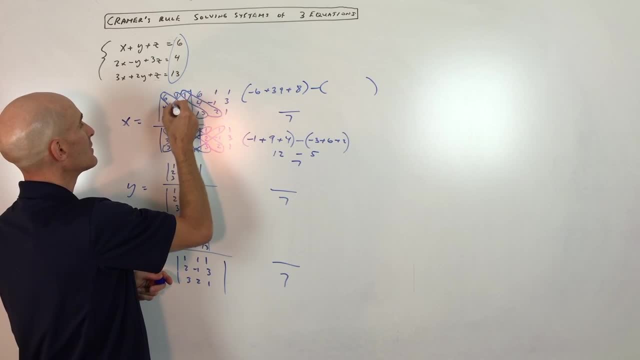 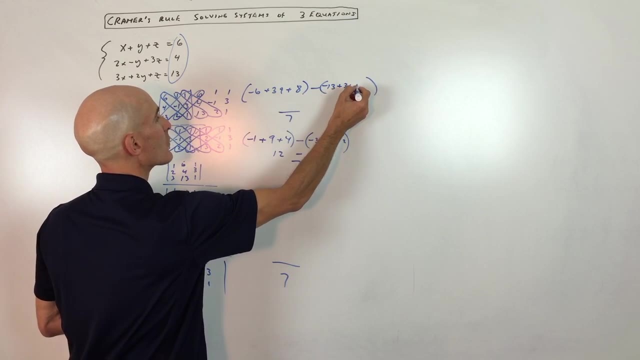 do the, we'll do the other diagonal. so, going up to the right now, that's going to give us negative 13. negative 13 2 times 3 times 6 gives us 36, so notice how we're adding those together. and then 1 times 4 times 1, which gives us 4, so that's 40 minus 13, which is 27. okay, over here we have what. 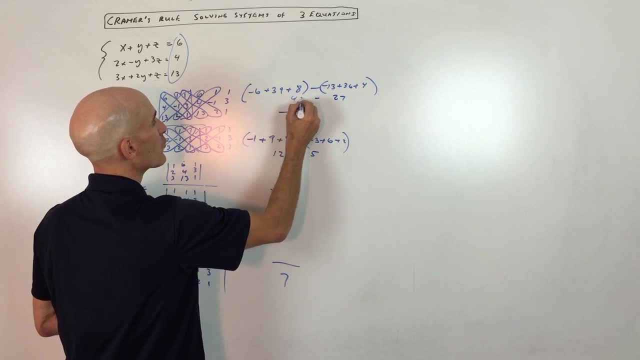 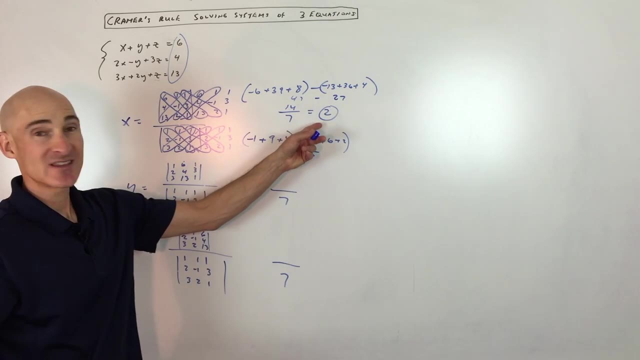 this is uh, 47 minus six, which is 41,, and 41 minus 27 is 14,, and 14 divided by seven is two. Okay, so that's it. so you got it, And you would repeat the same process for y and z. 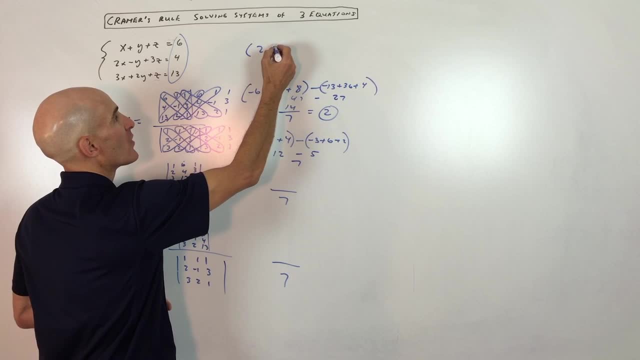 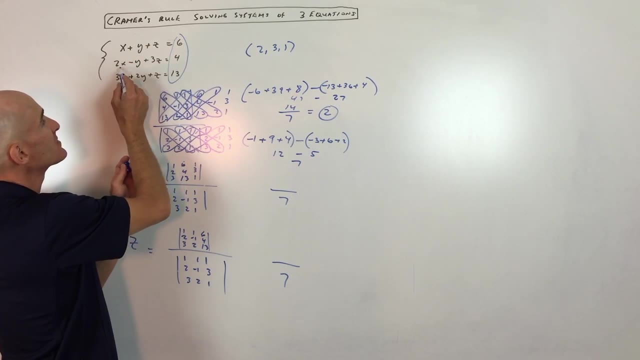 and then what you can do. once you get your answer, I'll tell you the answer for this one, if you wanna solve it. it should be two, three and one And you can check by putting it back in: Two plus three plus one is six. Put two, three and one, you should get four. Two, three and one, you should get 13.. 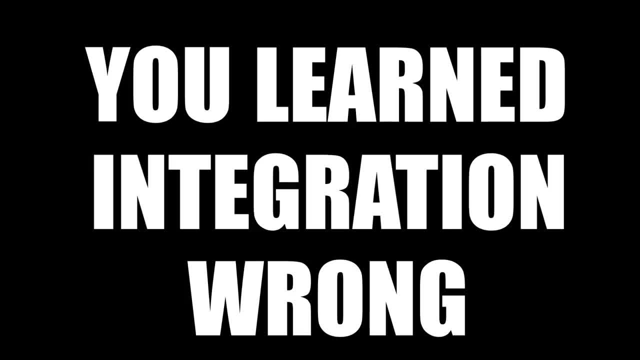 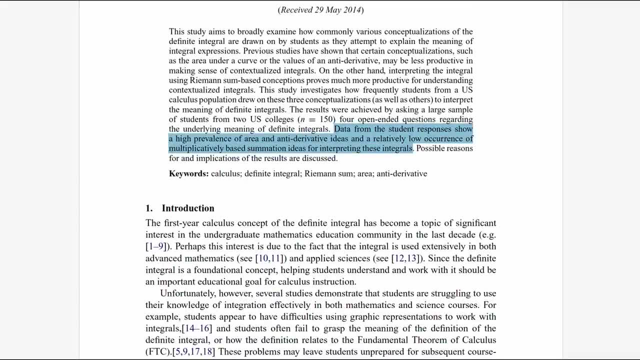 You learned integration wrong. That's quite a claim, so let me clarify what we mean by it. Our claim is based on studies of former calculus students that analyzed what students think. integration means Students tend to conceptualize integration to have one of three meanings.